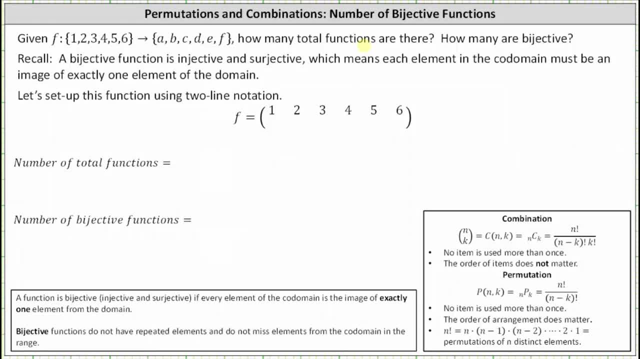 bijective Notice below. I've set the function up using two-line notation, where we have the inputs or elements from the domain in the first row. In the second row we will have the outputs or the elements in the range which must come from the elements in the codomain, which again is a set. 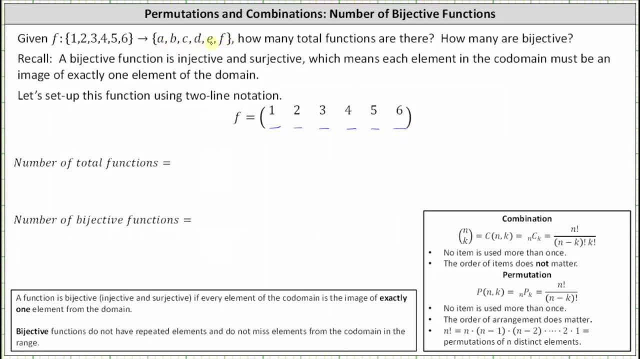 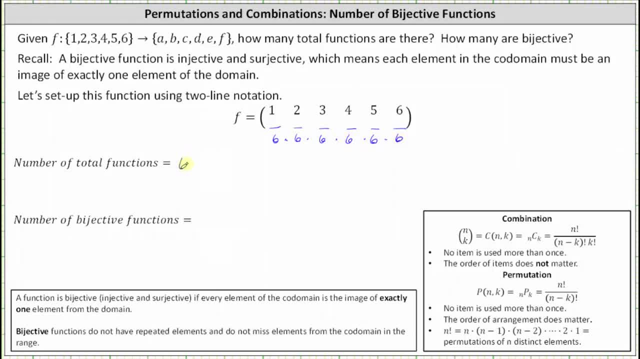 possible functions, Which gives us six to the sixth, which is equal to 46,656.. There are a total of 46,656 possible functions And now let's determine how many are bijective. Remember that a bijective function is injective and surjective, which means each element in the codomain must be an image of 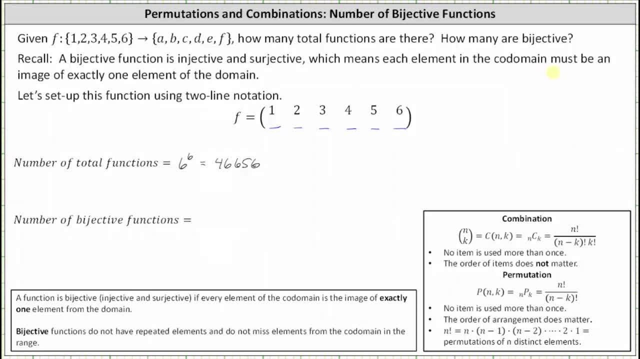 exactly one element of the domain. In order for a function to be bijective, the number of elements in the domain and codomain must be the same. Notice: in this case, both sets do contain six elements. There's a couple ways to approach this. Let's first use the multiplicative. 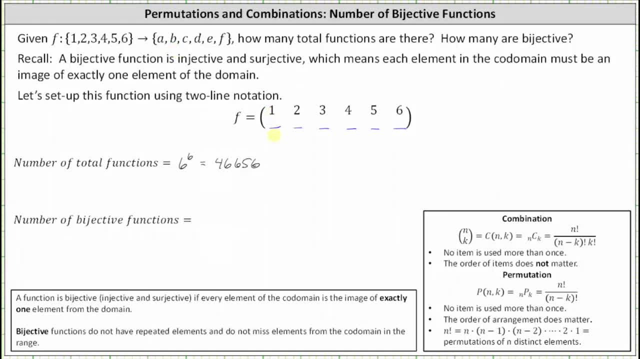 principle where, for the first input, there are six possible outputs, But then. but then because bijective functions do not have repeated elements and do not miss elements from the codomain in the range, there are only five possible outputs for the second input, followed by four possible. 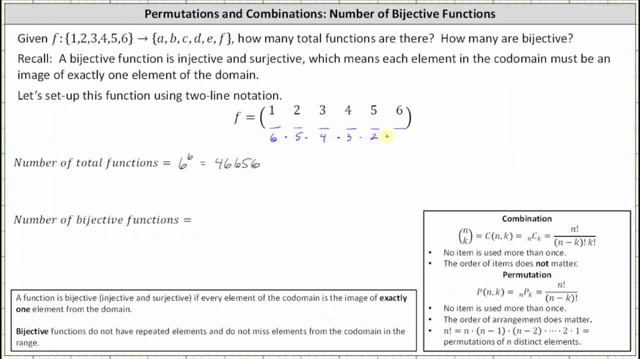 inputs for the third input, three for the fourth, two for the fifth and one for the sixth. Notice how no element in the codomain is repeated and no element from the codomain is missed in the range. Notice how the number of bijective functions is equal to six factorial. A second approach would be: 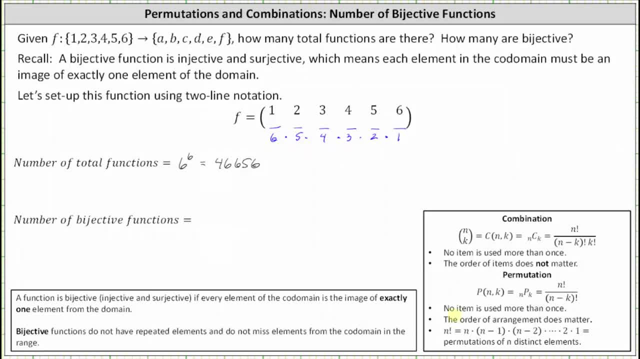 to use a permutation where- remember, for a permutation, no item is used more than once and the order of the arrangement does matter, Which means the number of bijective functions is also equal to the permutation of six items selected, six at a time, or six permute six.